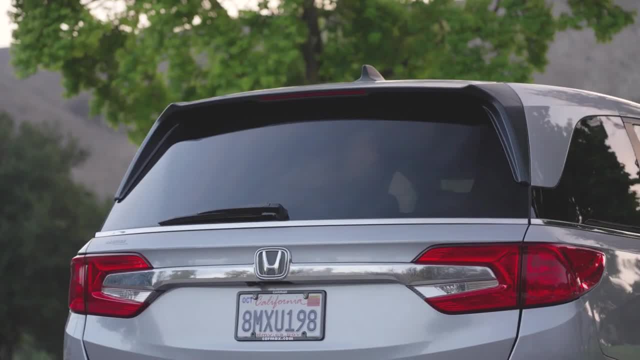 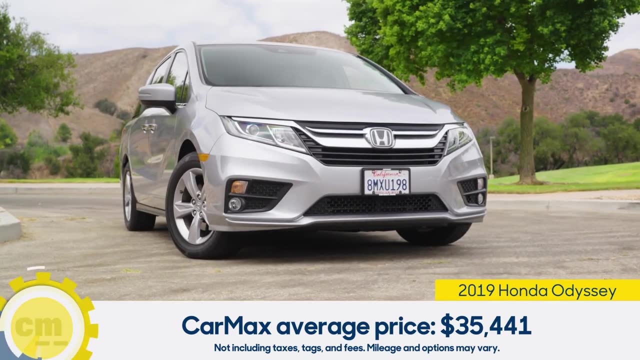 the second year that it was in production. It's known for two things: a clever interior and a composed drive. On average, CarMax sells 2019 Odysseys for a little over $35,000, depending on things like the trim. 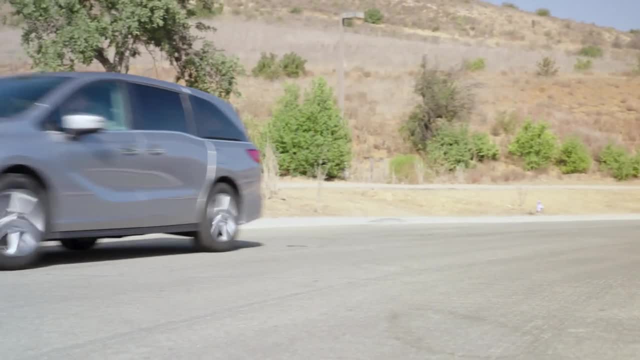 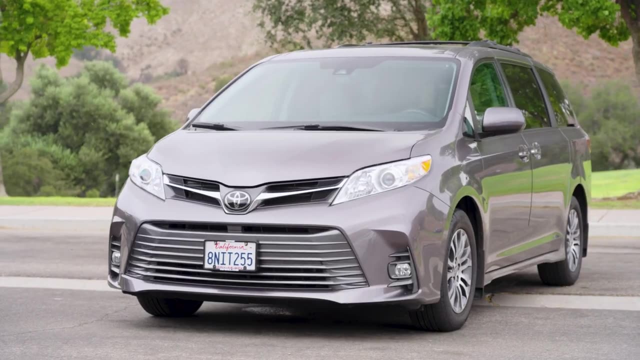 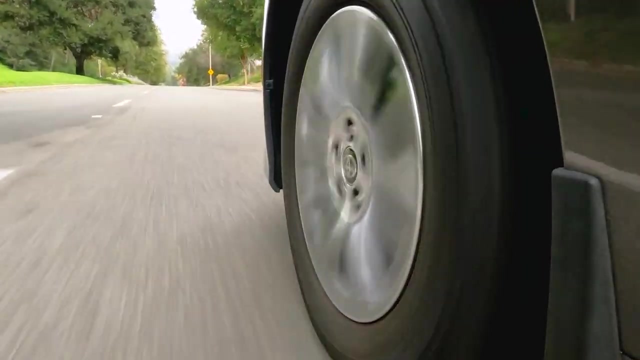 This Sienna is a little different. Toyota made this version from 2011 to 2020, which means this is the final year of the older generation. It's still impressive, and you're more likely to score a deal on one. CarMax sells the 2020 Sienna for an average of just. 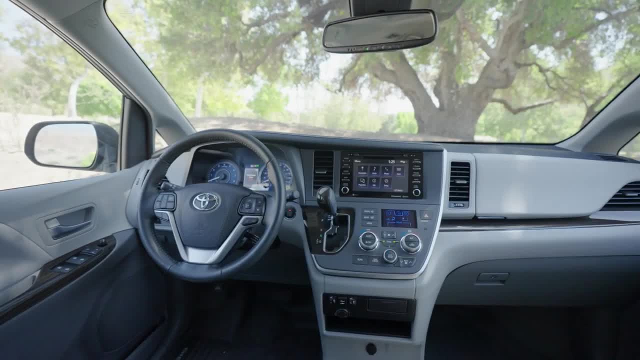 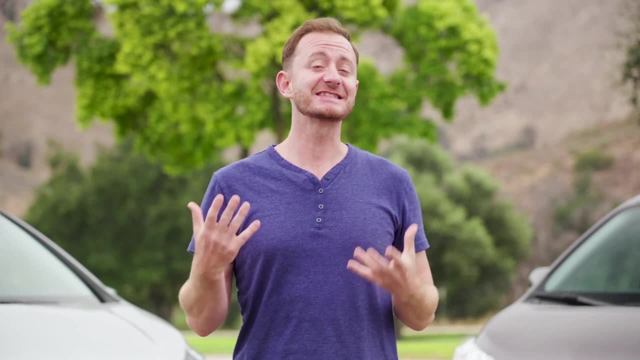 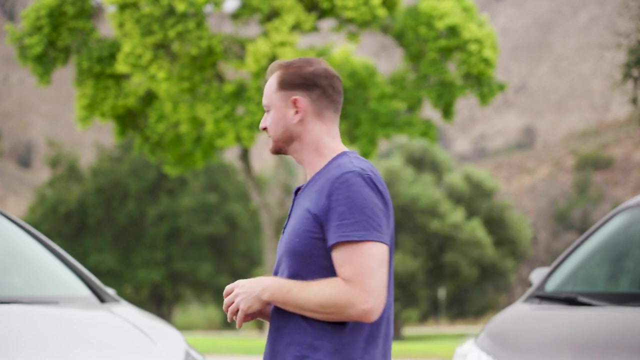 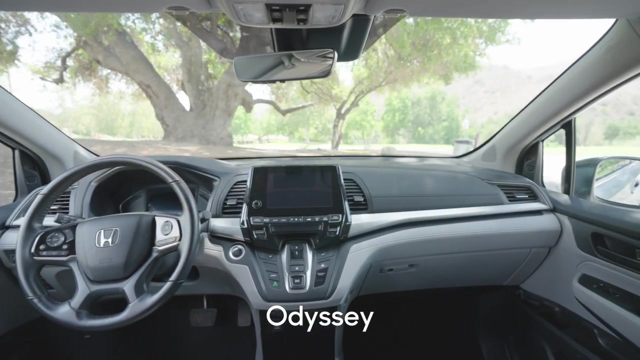 under $35,000, again depending on trim level, mileage options and other factors. Let's climb inside and see what this car has to offer. Honda has a reputation for solid construction, and this Odyssey is a good example I like. 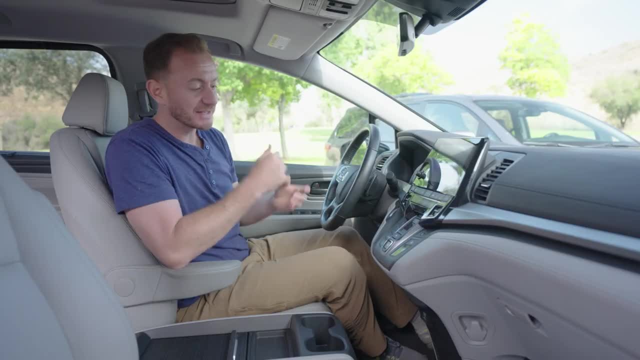 the materials like this soft dash, comfortable arm rests and even some cool plastics, which is not a given in some minivans. I like the materials like the soft dash, comfortable arm rests and even some cool plastics, which is not a given in some minivans. 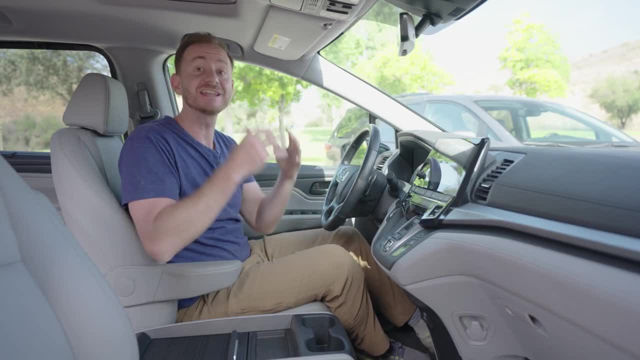 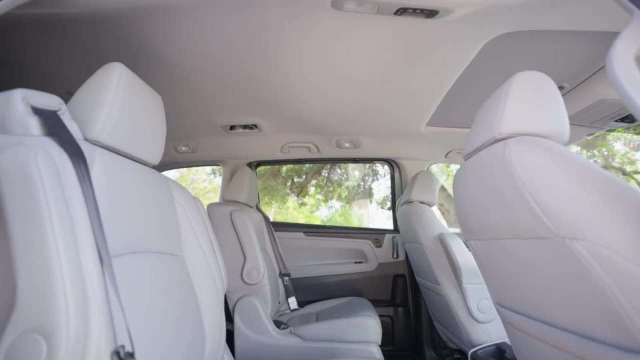 I like the materials like the soft dash, comfortable arm rests and even some cool plastics, which is not a given in some minivans. Actually, using the space is another strength. It is really roomy in here, Whether you're in the front row or the second or third, there is a lot of headroom and passengers. 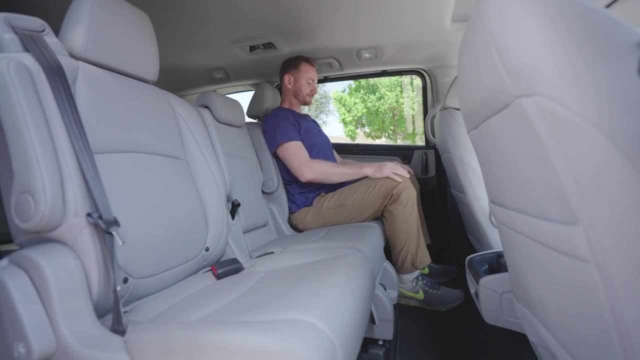 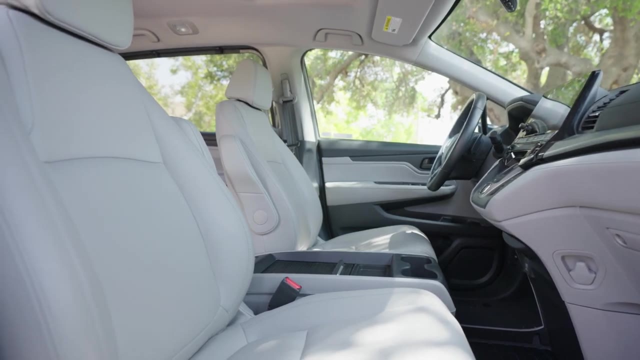 in the back can even stretch their legs out a bit. Now in our Edmunds testing, we found that the front seats are nicely cushioned and very supportive too, so they'll ease your stresses. Same goes for the second row. However. the third is a little bit cramped, so save that. 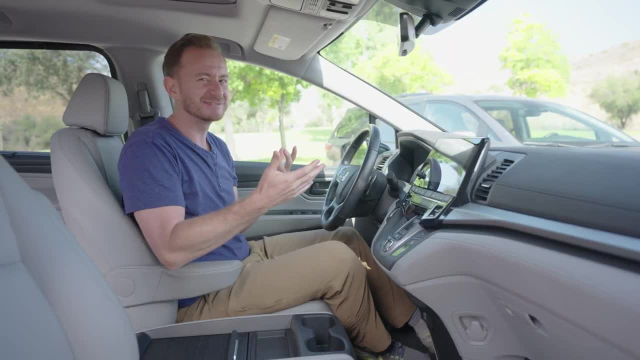 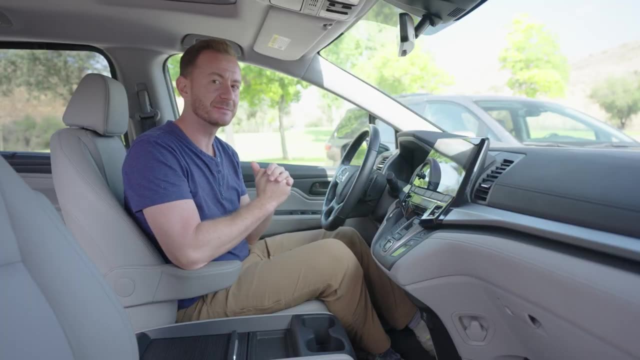 for short trips, Or that one friend of your kid's that you secretly don't like. Now, technology is the first place where the Odyssey slips up. Personally, I don't like that there aren't any physical buttons on the screen, save for this little volume knob. 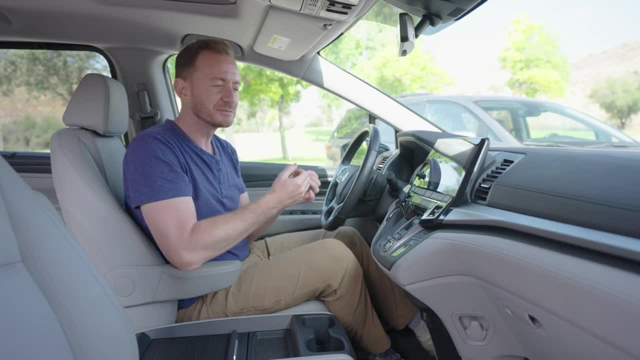 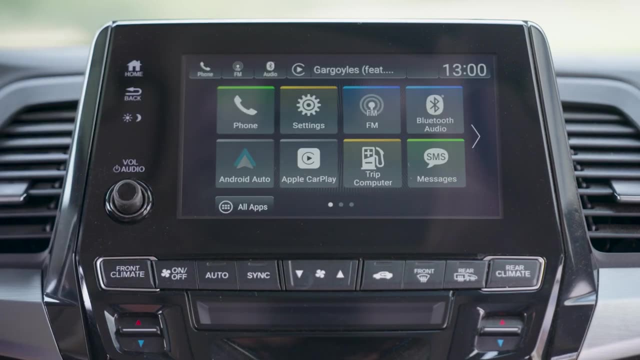 thankfully, And in our Edmunds testing we've noted multiple problems with the 8-inch screen that comes on the EX trim and up. Sometimes it will drop your smartphone connection, other times it will start glitching and sometimes it just goes completely dark. 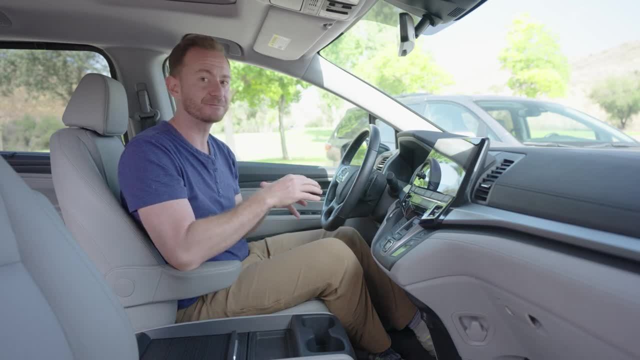 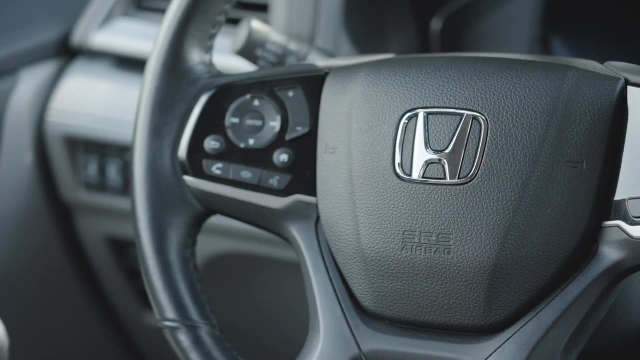 Now some models that you may find could have this worked out, so just be aware of it. We've also found that the voice controls don't understand you as clearly as those in some other systems. However, the intercom system that comes on some trims, that's pretty neat. 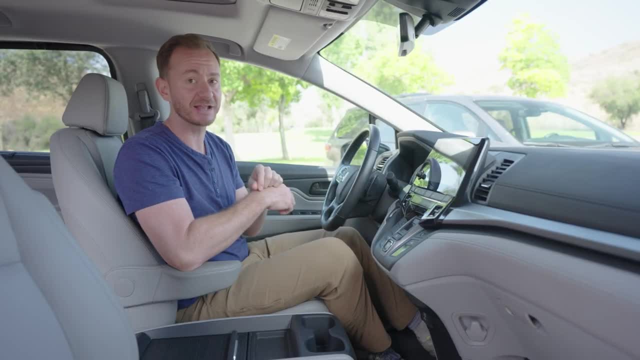 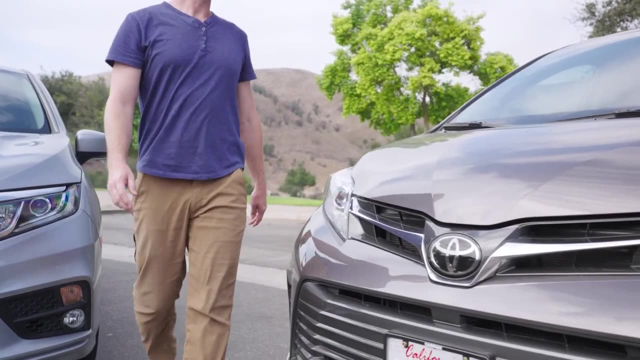 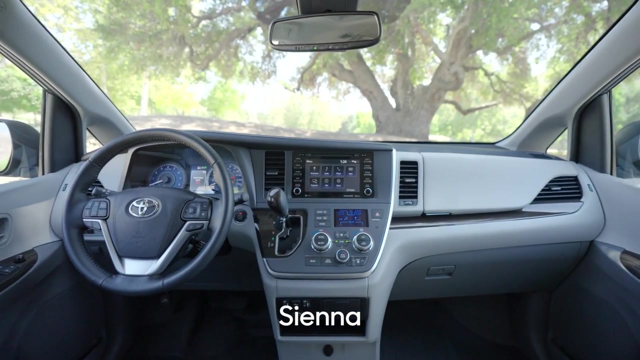 So look for the EX-L trim with navigation and the RES package if you'd like to get that. Now let's head over to the Sienna and see how that interior checks out. So yeah, Toyota did not take the same approach with its Sienna and I can't deliver the same. 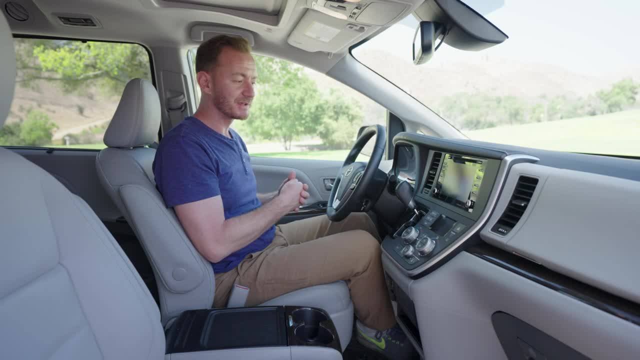 glowing verdict that the Odyssey got once we're inside. First of all, there's just a lot of hard material in here and this whole entire center area is basically plastic city. I mean sure it'd be easy to wipe and clean, but it's not looking real nice from where. 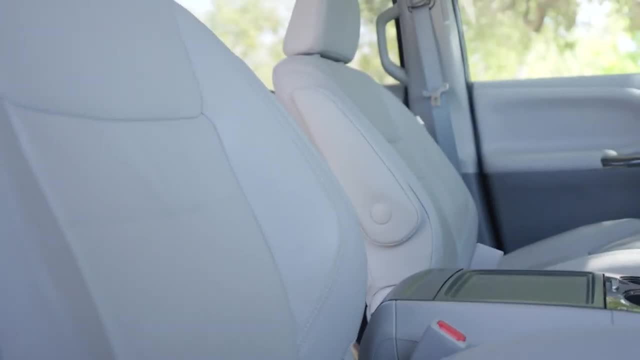 I'm sitting. Toyota did step up the cushiness, though with these leather seats, Feels like they're giving it away. Yeah, Yeah, They're giving me a hug. However, they fall a little bit flat when it comes to support. 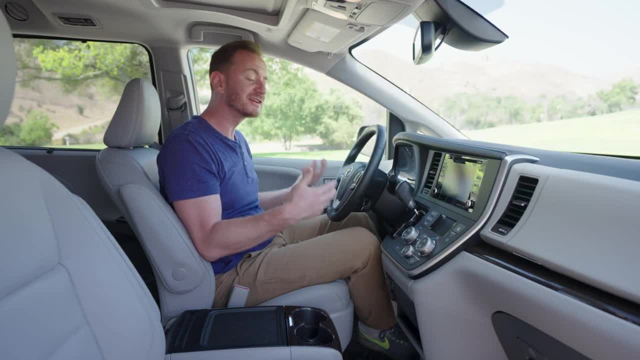 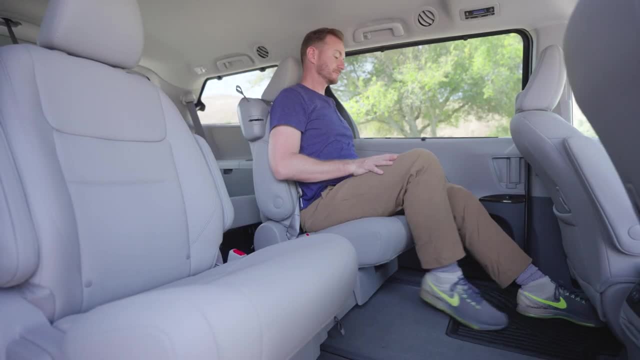 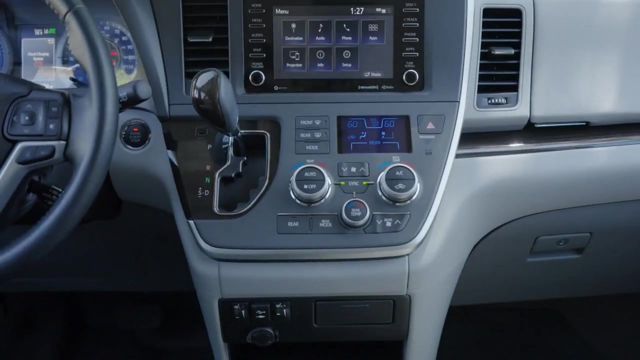 So on long trips, you and your passengers may find yourselves making a lot of adjustments just to stay comfortable. One plus side is that on upper trims there are available footrests in the second row. That's pretty sweet. Tech-wise, all Siennas come standard with a 7-inch screen, so you don't need to upgrade. 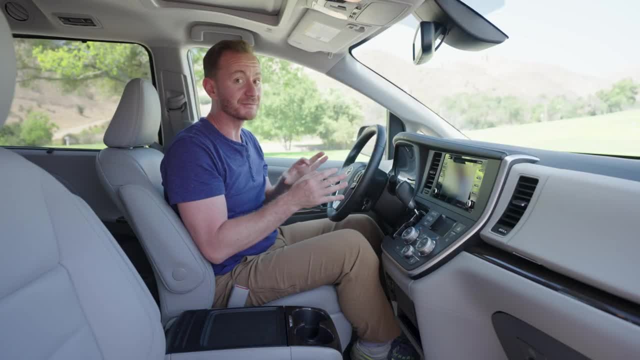 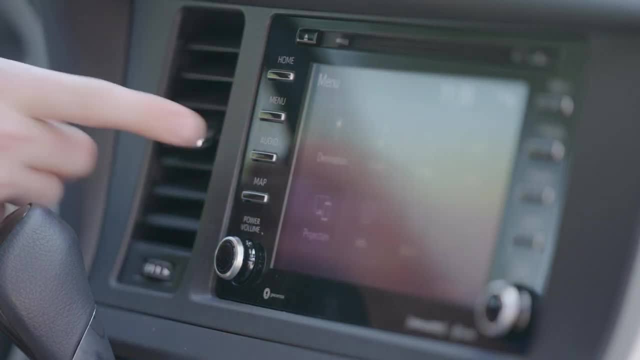 to get to a better unit or anything. It does work really well. There are just three things you need to know. First of all, the buttons are all really small, the graphics look pretty old and if sunlight catches it it washes the whole thing out and becomes really difficult to. 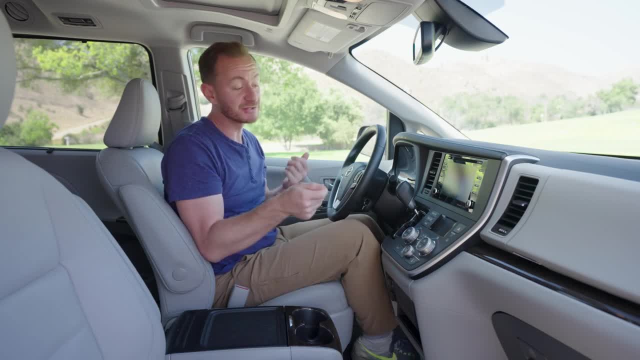 see Now, if you have an iPhone, it's very simple to just connect and boot up Apple CarPlay For you, Android users, though, sorry, but no Android Auto. Instead, you have to go through Toyota's mobile app called Entune and in our Edmunds testing. 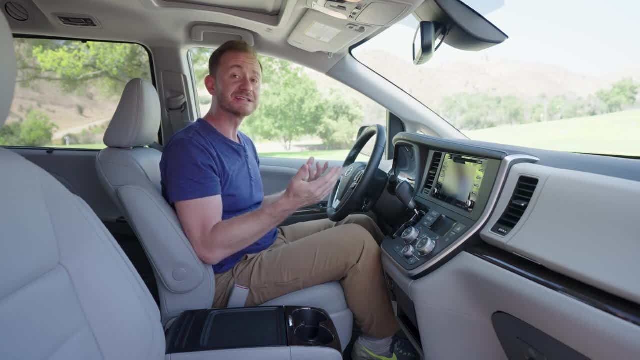 we have just never been fans of that app. On the plus side, just like in the Odyssey, there's an available intercom on upper levels of the Sienna, and that makes it pretty fun to play tricks on your kids in the back. 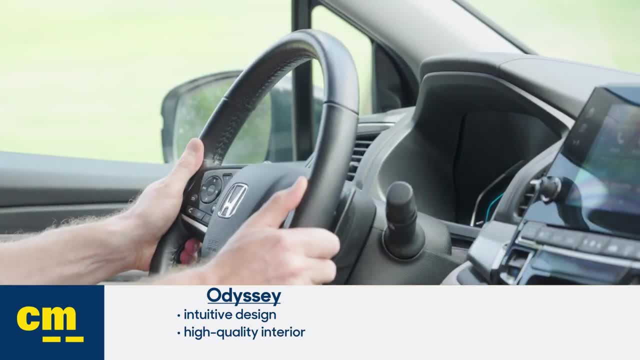 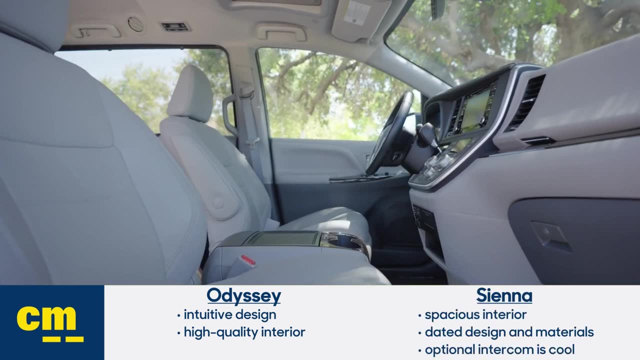 The Odyssey interior is the better choice. I find it more intuitive and more dressed up. If I'm going to be in a minivan, I want to feel like I'm being rewarded for the decision. Now. there is plenty of space in the Sienna, but it seems like there are lots of barriers. 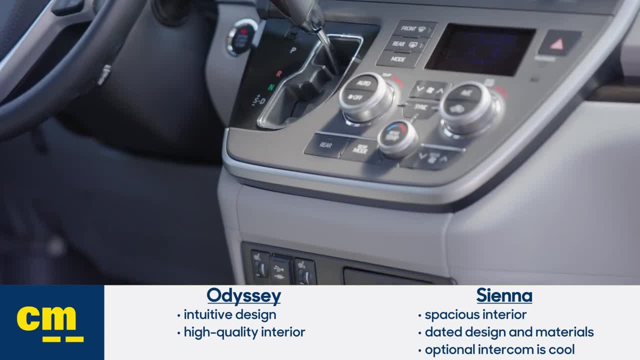 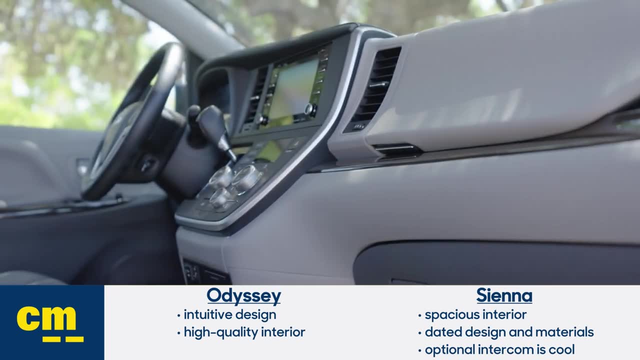 to drag it down, whether that's downgraded materials or a screen that feels about five years older than it is. A cool intercom is more widely available in the Sienna than in the Odyssey, but it's not enough to save it. But what about behind the wheel? 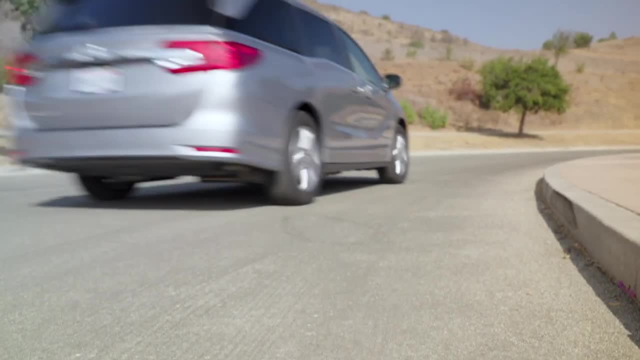 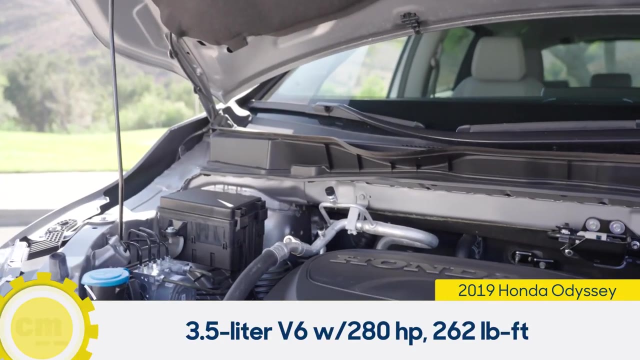 See how these two behave once we get them on the road. What if you stretched a sports sedan into a minivan, The Honda Odyssey? Under the hood, you get a 3.5-liter V6 engine and it has no trouble getting up to speed. 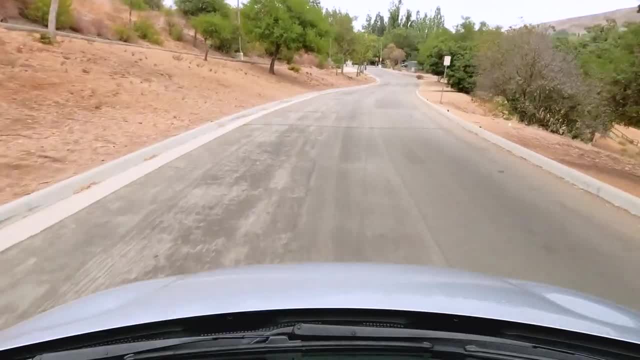 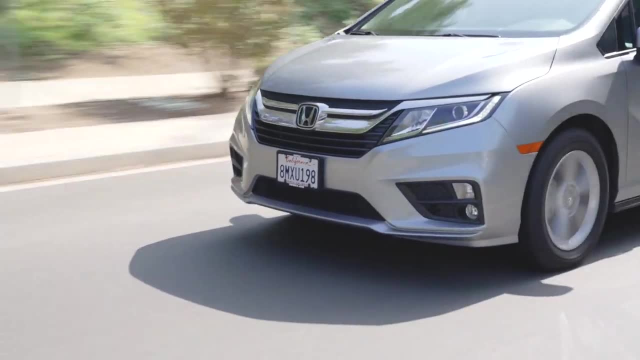 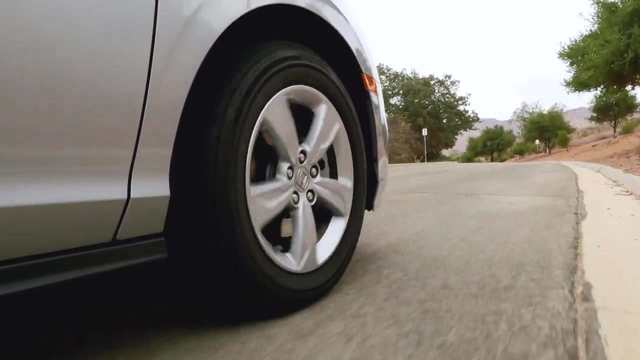 The Odyssey has a firm suspension for a minivan. That makes it ride a little rough over bumps in the pavement but it also results in handling that is pretty shocking for a van and can clearly handle curves better than the rest of the class. Stick with the 18-inch wheels, because we've found the 19s on the Elite trim are not advisable. 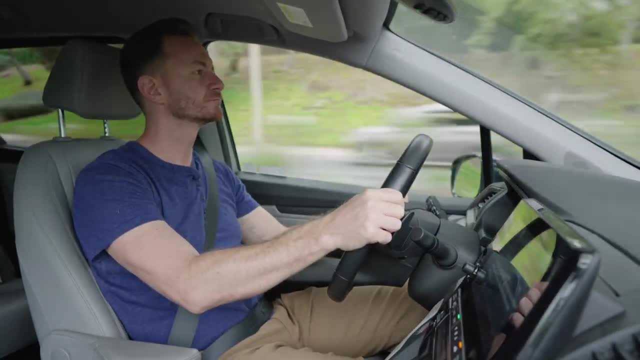 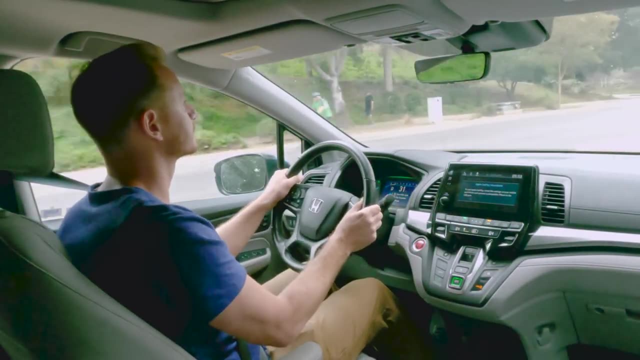 for people sensitive to ride comfort. The Odyssey glides with impressive quiet inside the cabin. Honda used insulating glass windows to keep the noise out. You know, as long as you don't have chaos in the back seats. We also like the transmission. 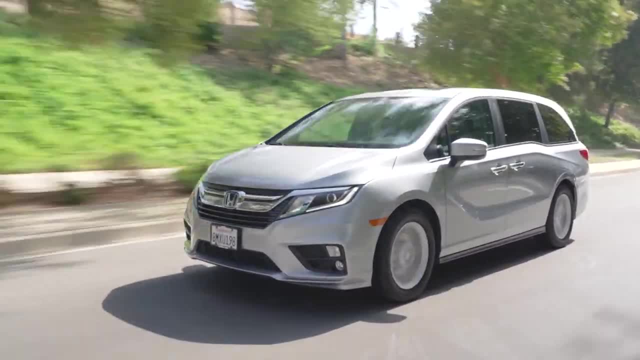 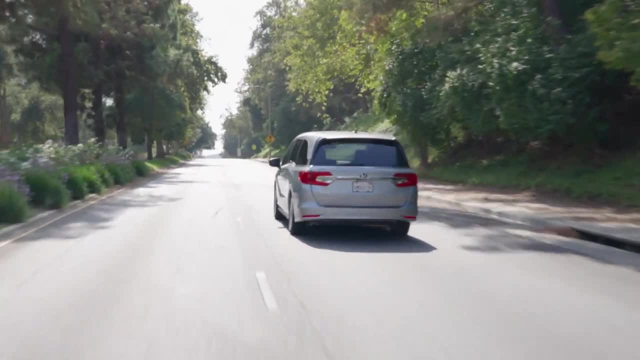 You don't have to worry about that. You don't have to worry about that. You don't have to worry about that. You can shift down for power or ease into better efficiency when you need. It stays out of the way. a good thing. 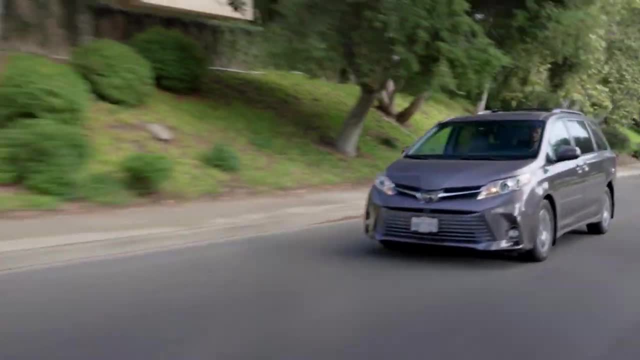 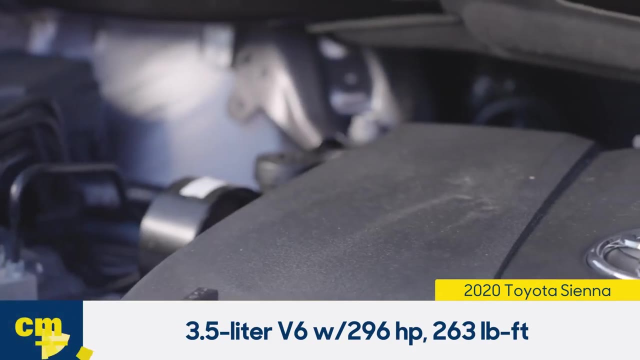 The Sienna has a lot going for it, but can it put all the pieces together on the road? Just like the Odyssey, this van has a 3.5-liter V6 engine. that is not wanting for power. This baby feels lively. 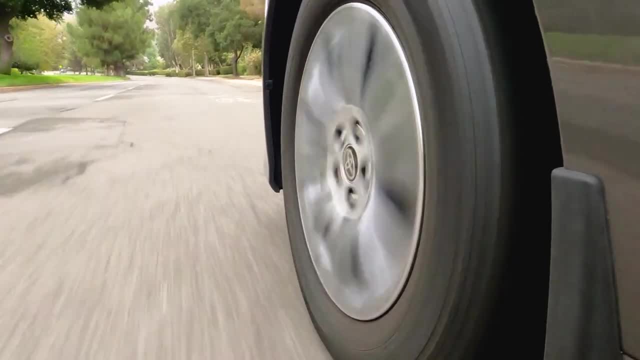 And available all-wheel drive is a big advantage. Things get messy elsewhere, though. The Sienna wants to be smooth and doesn't leave a spot, And thanks to the unique steering system, this is a perfect choice for a very floor-to-ceiling car. 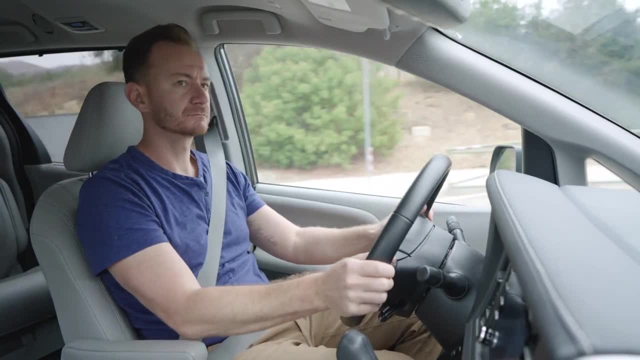 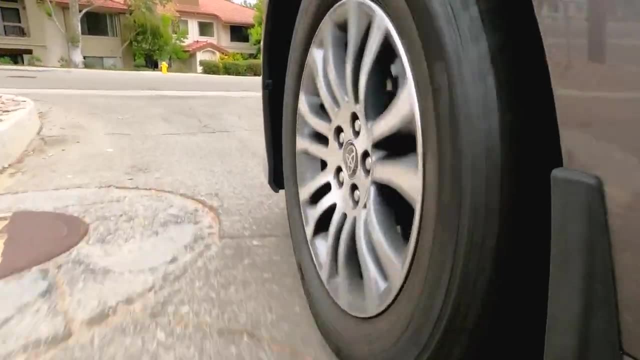 doesn't like dynamic driving. The steering is light, meaning you don't get much feel for the road. The body moves around under hard turns. Now the brakes feel pretty good, Not as strong as the Odyssey, but confident. The Sienna is easy to drive, but it just. 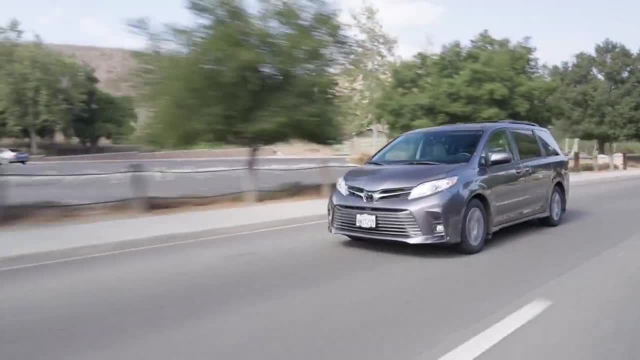 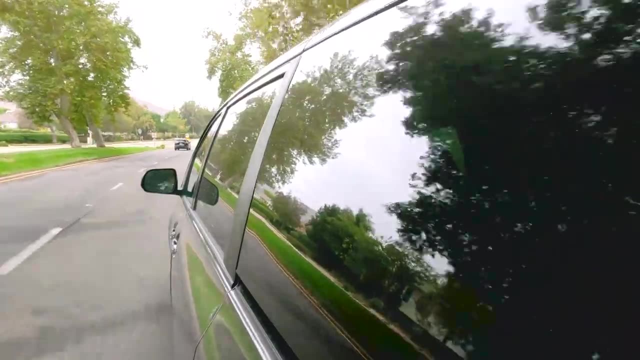 isn't as cohesive an experience as the Odyssey. The transmission is a great example. It's an eight-speed automatic and from time to time it's not in lockstep with the engine. Sometimes it's jumpy, sometimes too laggy. 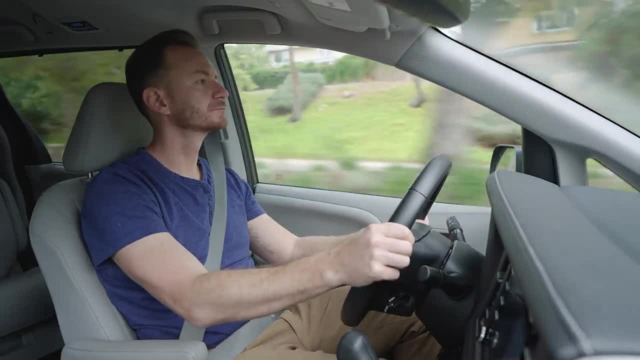 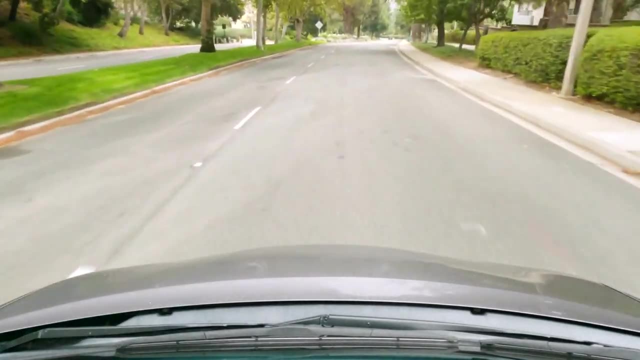 Sadly, it struggles to find a rhythm. The Sienna is simply more comfortable than the Odyssey on the road, however, Its suspension handles bumps and cracks really well during our Edmunds testing, ensuring you won't feel much disturbance inside. This is a cloud-like experience. 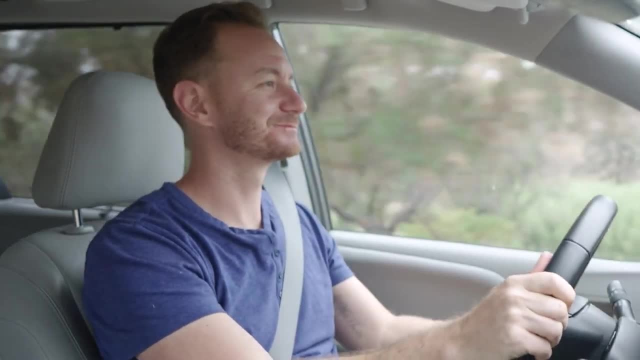 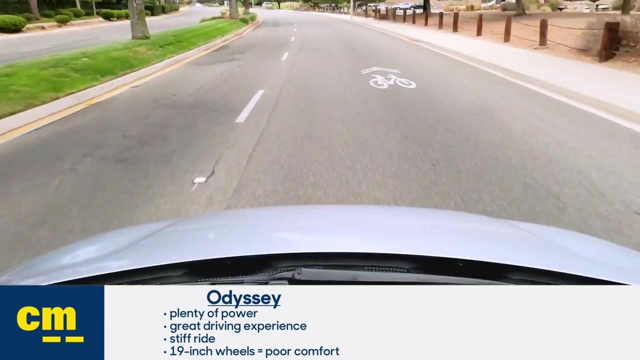 You deserve that. You're doing great. Honda has the clear winner here. The Odyssey does everything you'd want in a minivan. It has the power you need and a surprising deftness to it everywhere else. Sure, a little extra comfort would help. 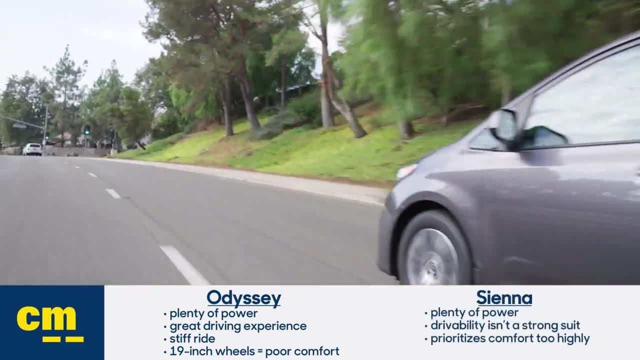 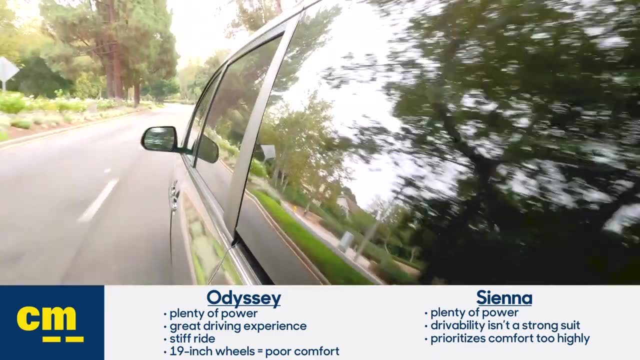 but behind the wheel it's a gem. The Sienna isn't going to be for everyone. Speed isn't an issue, but the rest of its driving performance sadly is. It just doesn't feel very focused or precise. on the road You get superior comfort, but it doesn't. 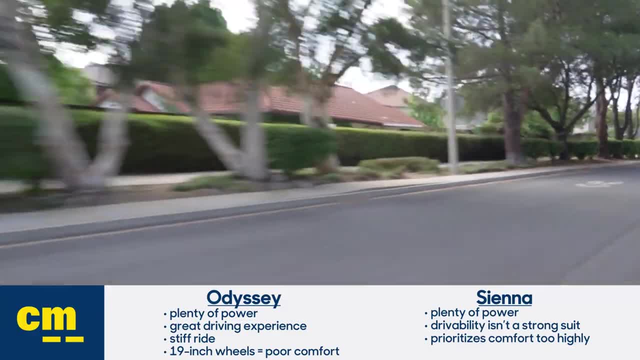 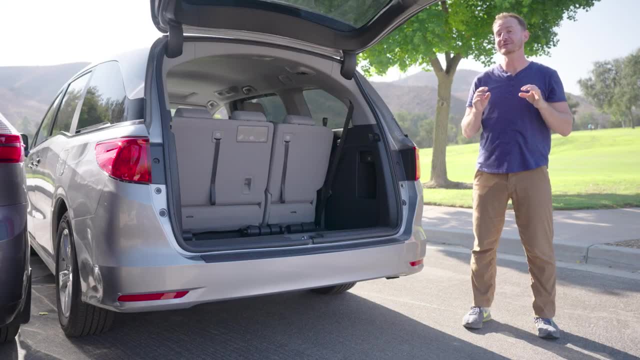 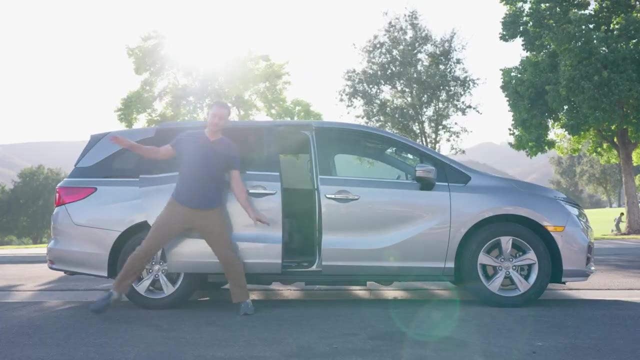 paper over the Sienna's flaws. Minivans have hidden tricks galore. Here's how to make the most out of the Odyssey. First, look for the EX trim and up. That way you get power doors that slide to the left. 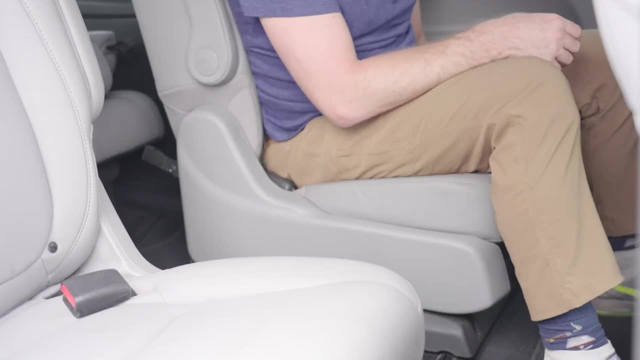 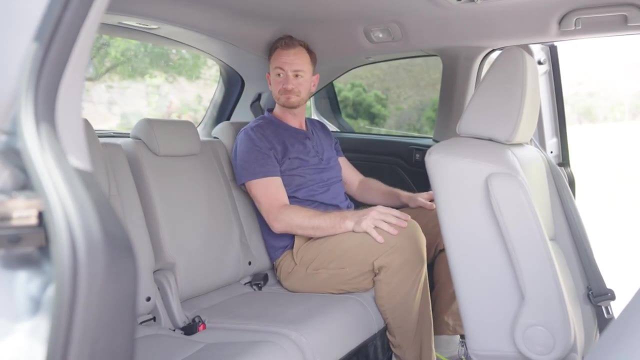 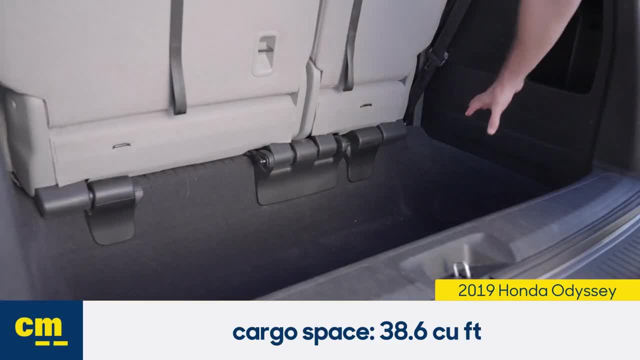 The Odyssey offers a lot of cargo space, and this underfloor storage helps a lot too. The Odyssey offers a lot of cargo space, and this underfloor storage helps a lot too. You can drop the third row down there like this. 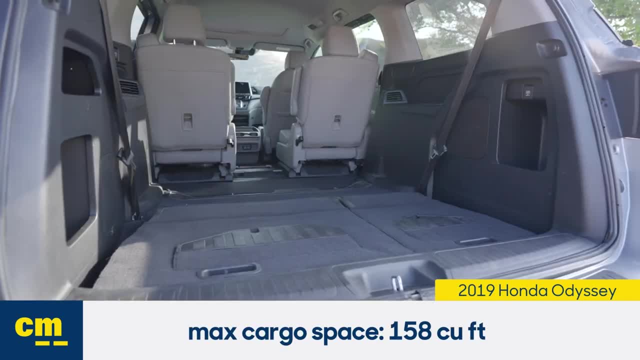 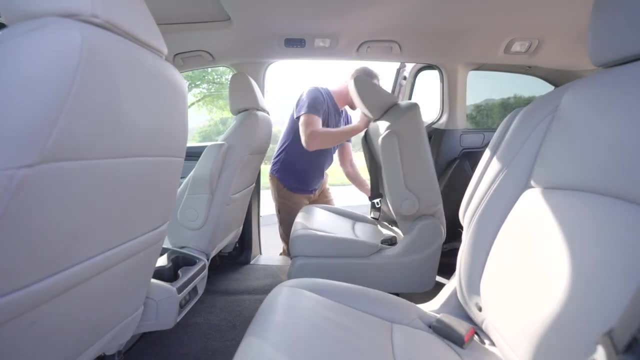 It isn't power but it's easy to do. The LX and EX trims get the most space behind the first row. Unfortunately, the second row is tough to remove, so don't plan on doing it a ton. Unfortunately, the second row is tough to remove, so don't plan on doing it a ton. Unfortunately, the second row is tough to remove, so don't plan on doing it a ton. When it comes to fuel economy, the Odyssey is not our favorite. When it comes to fuel economy, the Odyssey is not our favorite. Not our favorite. 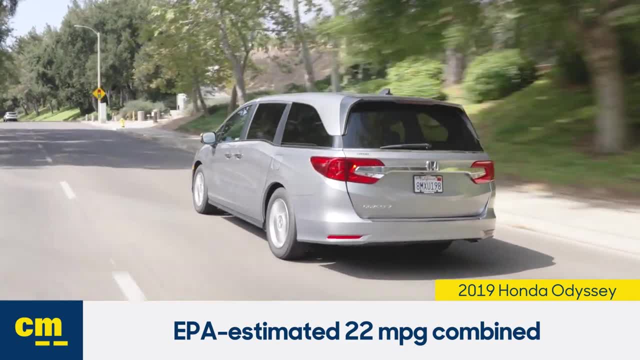 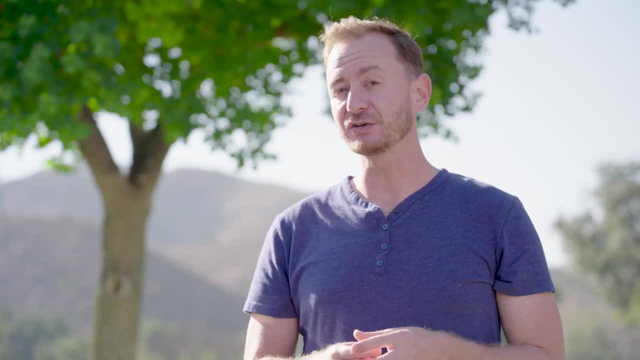 Its ratings are fine on the surface. An EPA-rated 22 MPG combined is right in line with other front-wheel drive minivans. But on our Edmunds evaluation loop the Odyssey underperformed that number. So just consider your driving style before buying one. 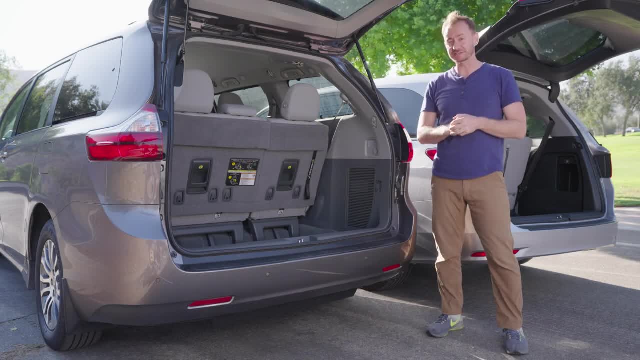 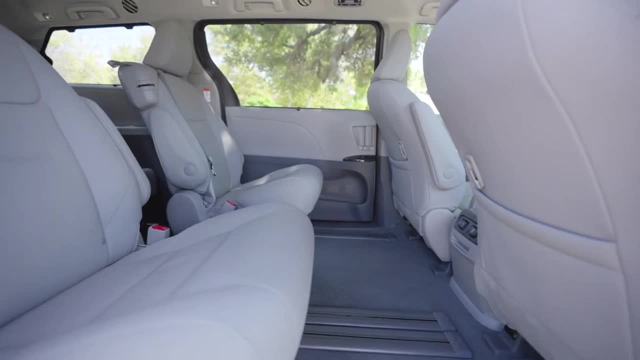 Not to be outdone. the Sienna has a few of its own strengths For power, sliding doors. on the Sienna you want the LE trim or up. And speaking of sliding, it's a big plus here because the second row rolls all this way back or forward. 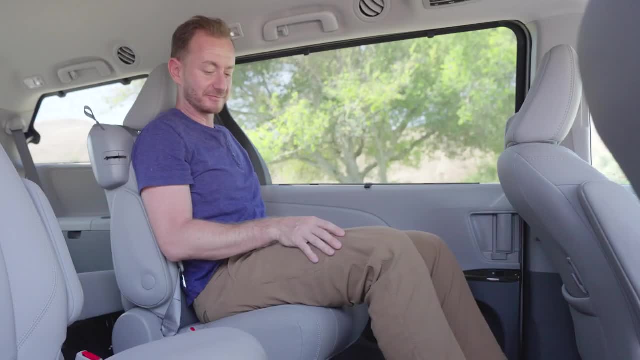 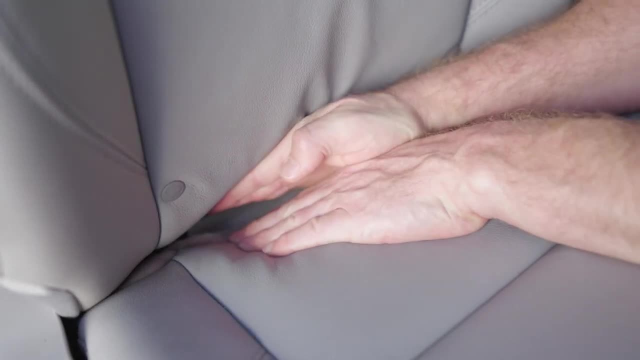 creating easy access and as much leg room as you need For car seats. you can leave them installed while sliding the second row, which is cool. Finding the anchors is easy, but the leather around them is hard to move And the tethers are hidden. 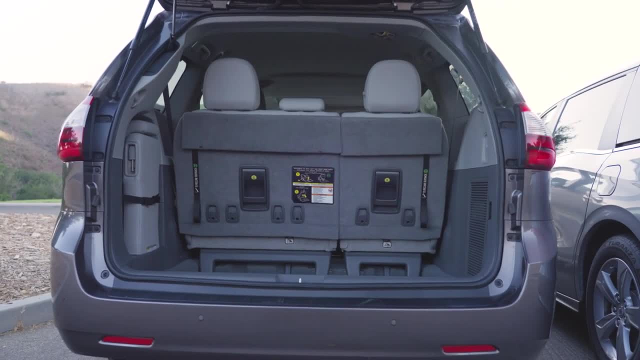 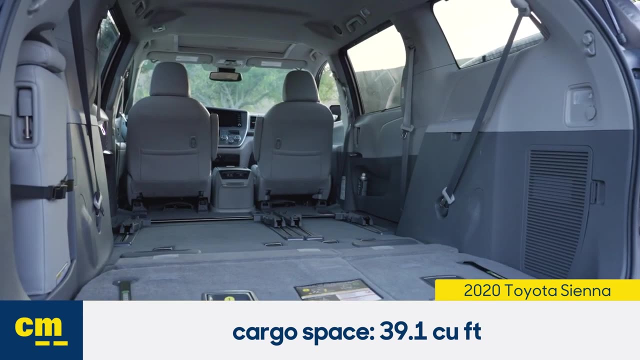 I wouldn't want to deal with that over and over Cargo time. The Sienna is a stellar choice. There is plenty of room behind the third row. The load floor is nice and low and almost completely flat when folded. There's good space behind the front row too. 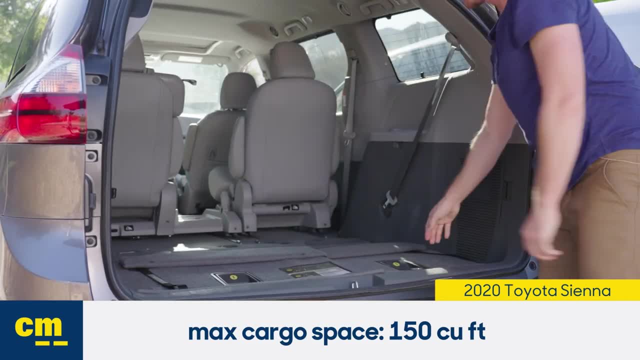 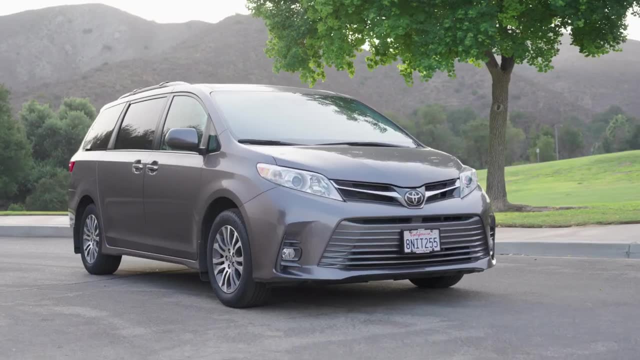 but still less than the Odyssey. However, the Sienna makes it pretty easy to remove the second row seats like this. They're heavy but I'm incredibly strong, So it's cool. At the pump, the Sienna fared better than the Odyssey.